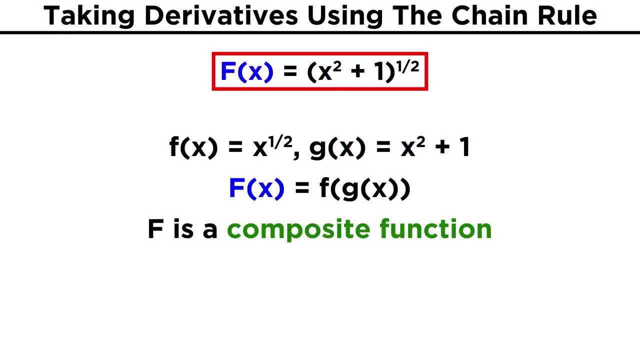 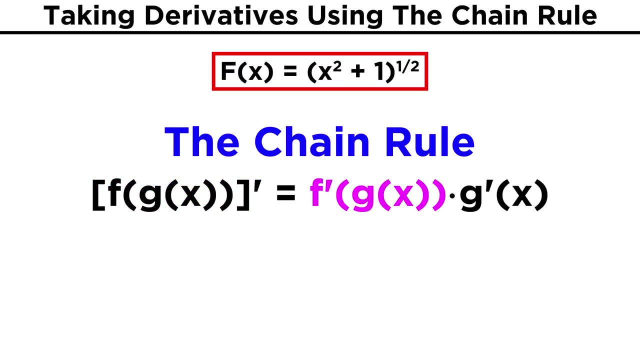 one. And if we call the composite function capital F of x, in trying to find the derivative of capital F of x, we are actually facing the same problem: trying to take the derivative of f of g of x. The way we do this, according to the chain rule, is that we find f prime of g of x, and 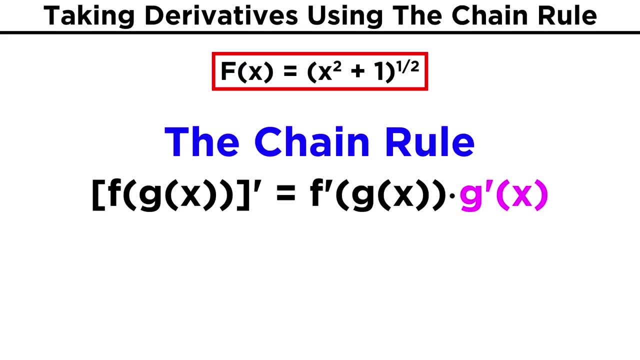 then multiply it by g, prime of x. What that means is that, moving from the outside in, we can take the derivative of the function as though this exponent is the only operation, leaving the inside as it is. But since the inside is another function, we have to multiply our result by the derivative. 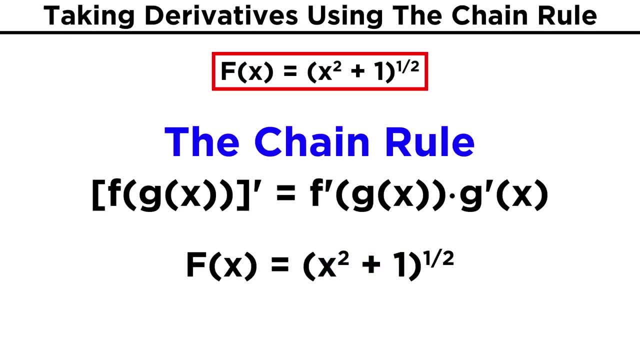 of what's inside. So, looking at x squared plus one to the one half power, let's apply the power rule Now. we are used to using the power rule for positive integer exponents, but don't worry, we can do this with fractional exponents too, and it won't be any different. 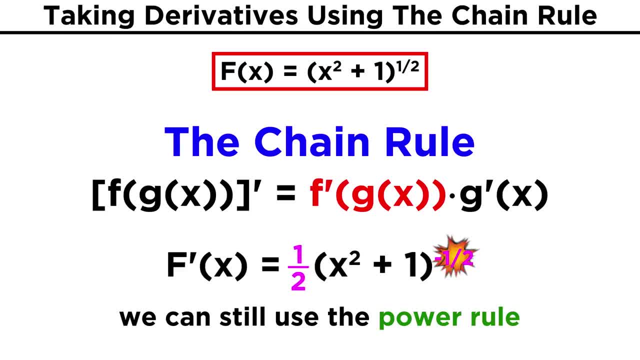 We just take the exponent and bring it to the front and then subtract one from the exponent, so we get one half times this parenthetical term which is now raised to the negative one- half power. If we recall our rules of exponents, raising something to a negative exponent is the same. 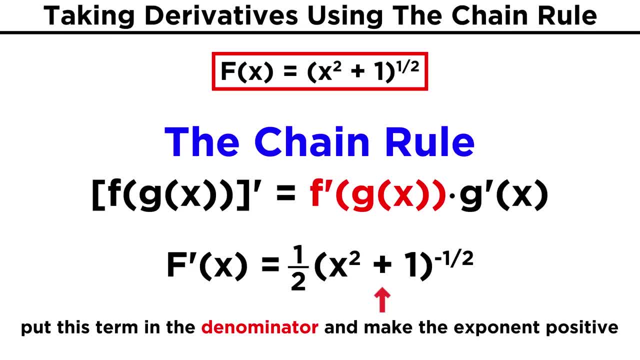 as one over that thing raised to the positive version of that exponent. so this becomes one over the quantity x squared plus one to the one half power, and we know that this simply means the square root of one. So we can go back to expressing this as root x squared plus one. 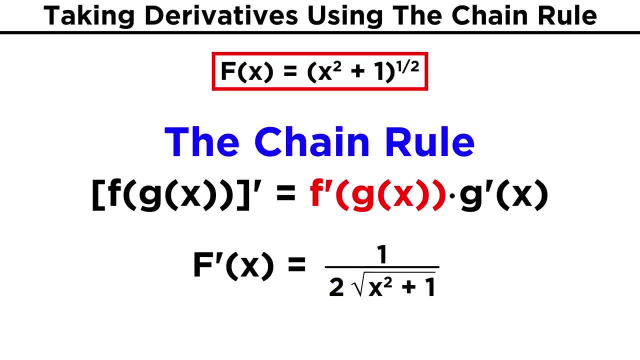 Incorporate the one half by putting two in the denominator, and this is what we get. But now we must remember: according to the chain rule, we have to multiply this by the derivative of the function inside the parenthetical as well, and the derivative of x squared plus. 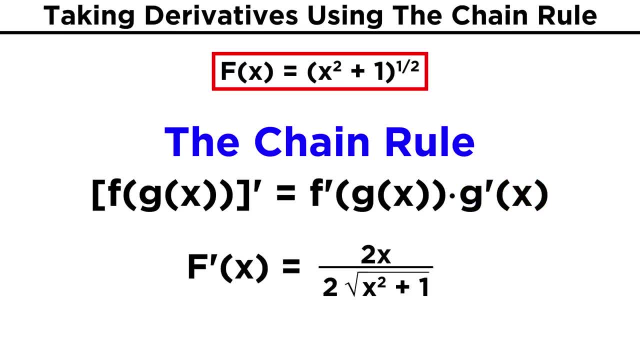 one is two x, So let's put the two x up top, Cancel out the two and we are left with x over root, x squared plus one. So with the chain rule, when we have multiple functions happening at once, we differentiate the outer function first, as it operates on the inner function, and keeping the inner. 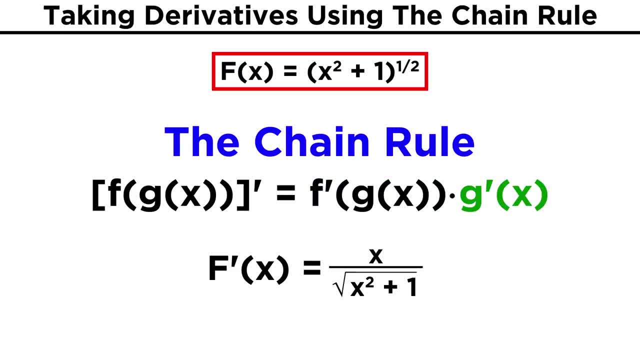 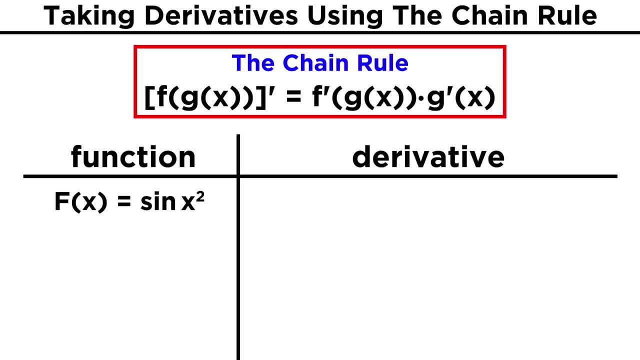 function the same and then we multiply by the derivative of the inner function. Let's try a few more for practice. Say, we want to get the derivative of sine of x squared. So we can clearly see that here there are two functions operating on x. 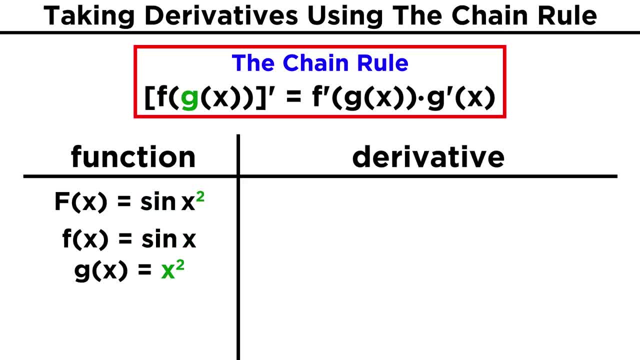 The outer function is sine and the inner function is this exponent. So let's apply the chain rule. The derivative of sine is cosine, so we get cosine x squared, But then we have to multiply by the derivative of the inner function, x squared, which gives 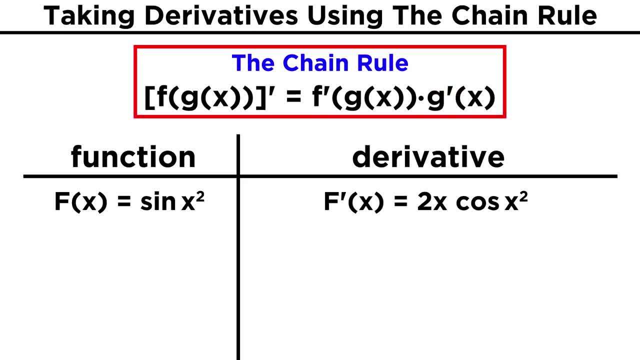 us two x, so we get two x cosine x squared. Just to see the reverse scenario: what if we have sine squared of x? Let's recall that this notation implies that the function sine of x is being squared. so we can also express that like this, with sine x, in parentheses, being raised to the. 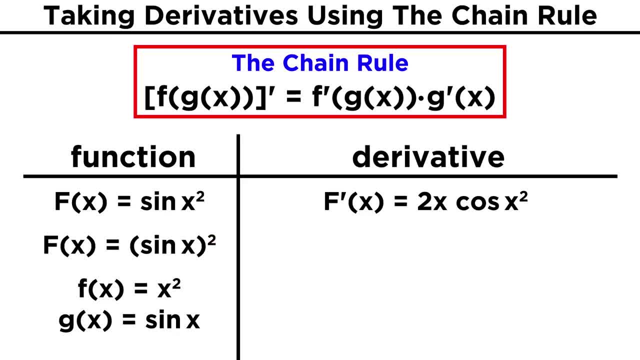 second power. Now the situation is reversed and the outer function involves squaring the input, while the inner function is sine. So we can also express that like this, with sine x in parentheses being raised to the second power. So let's take the derivative of the outer function, which means pulling the two down. 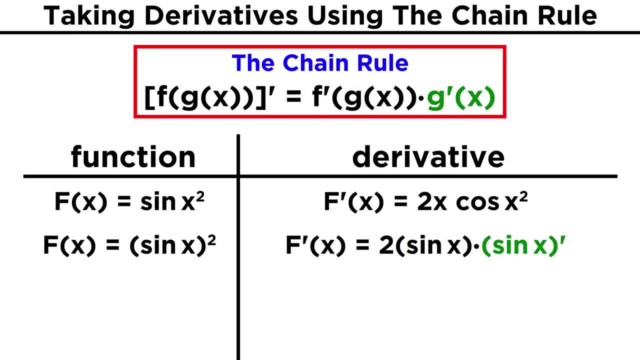 here to get two sine x. But then we multiply by the derivative of the inner function, and the derivative of sine is cosine, so we get two sine x, cosine x. Apart from good practice, these two examples should also prove to you that it is indeed. 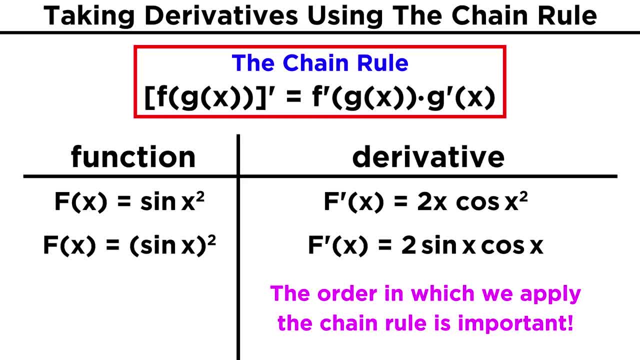 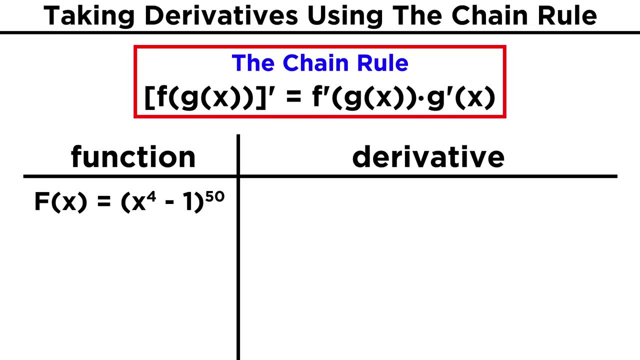 important the order in which we apply the chain rule, as we do get different answers. It's the derivative of the outer function as applied to the inner function times the derivative of the inner function. Now let's try some other examples. Take the quantity x to the fourth, minus one raised to the fiftieth power. 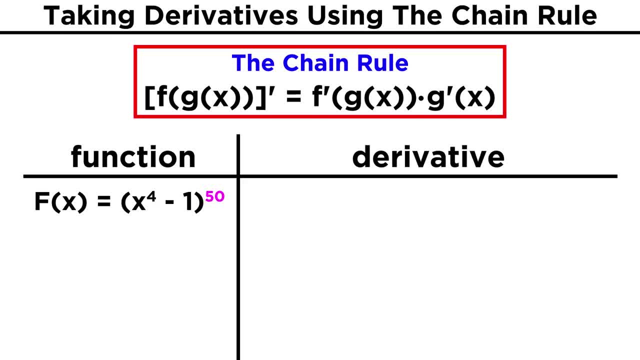 This huge exponent might seem daunting, but let's just apply the chain rule. The outer function is this exponent, so we take the fifty and put it down here. leave what's inside the parentheses down here. Leave what's inside the parentheses down here. 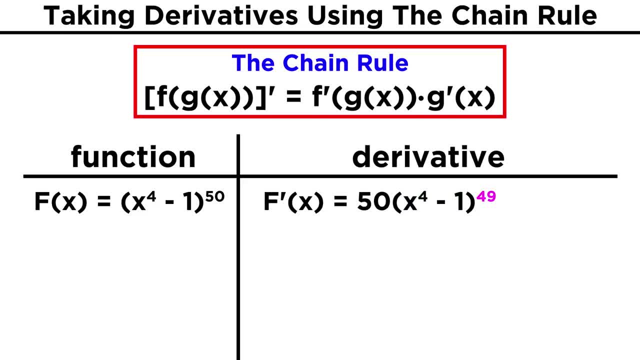 Just as it is and reduce the exponent to forty-nine. This is no different than what we are used to, But then we multiply by the derivative of the inner function, and that will be four x cubed. So combining these terms, we get two hundred x cubed times the quantity x to the fourth. 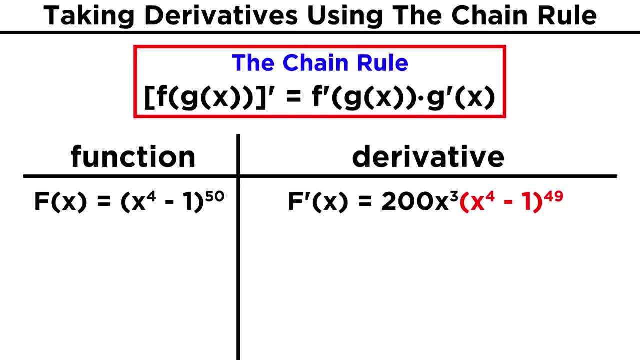 minus one raised to the forty-ninth power. A little messy perhaps, but not difficult at all. However, there are instances in which we will have to combine the chain rule with the product rule or quotient rule. Take, for example, x minus one over x plus one quantity squared. 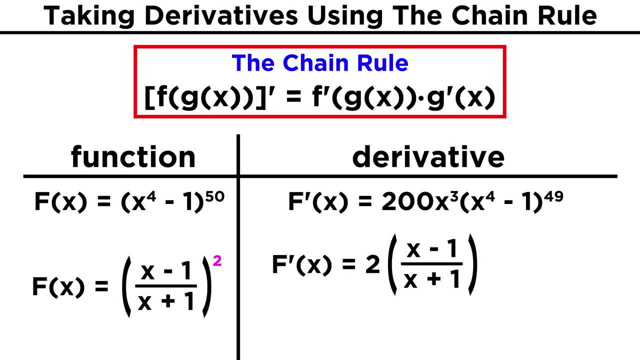 Naturally we need the chain rule. We take the derivative of the outer function and we get two times this parenthetical. But now we must multiply by the derivative of the inner function and to do that we need the quotient rule. 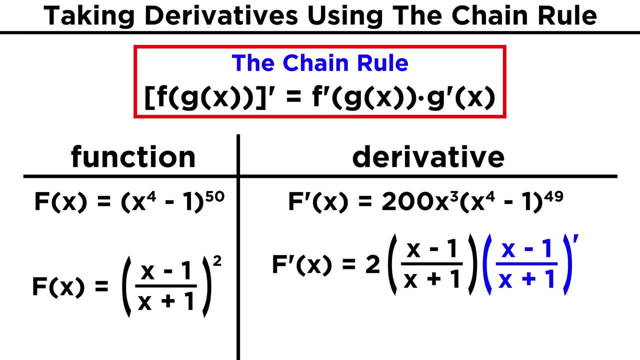 Let's save our place in this problem so that we can come back to it once we find this other derivative and set up our quotient. That will be x plus one times one minus x minus one times one over x plus one quantity. 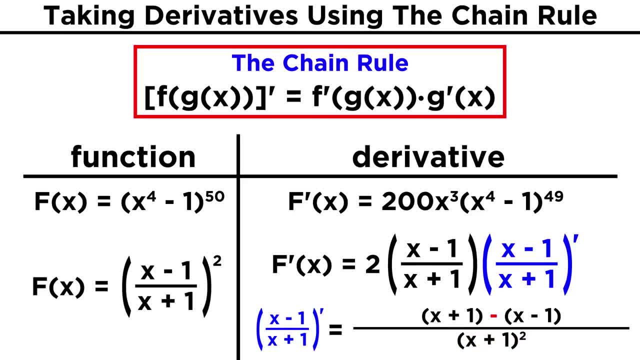 squared. Simplifying the top and being careful to distribute this negative sign, we get two over x plus one quantity squared. Now, since this is the derivative of this quotient, we can plug this in back here where we needed it. 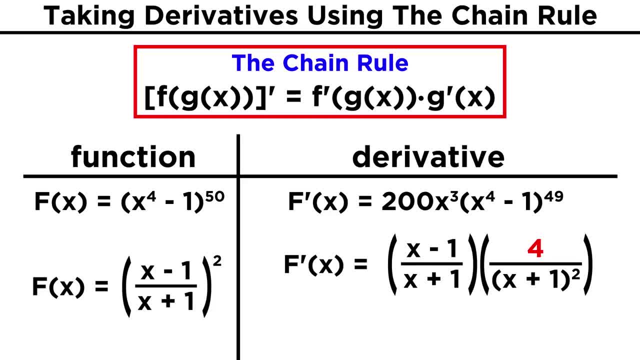 We can simplify by combining the twos in the numerator to get four, and since the denominators have the same term, let's just make this x plus one quantity cubed, And that's pretty much all we can do. Let's try another. 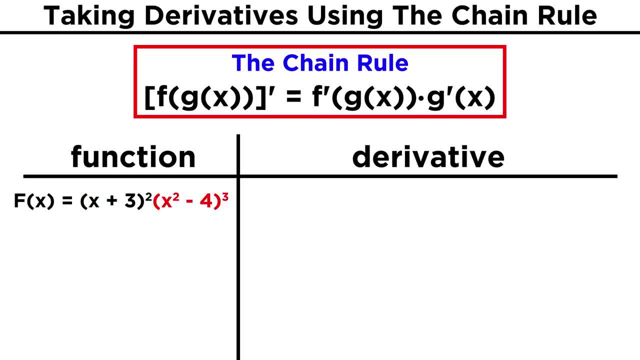 X plus three, quantity squared times x squared minus four, quantity cubed. This time we will have to use the product rule and the chain rule, but we will have to use the product rule first. This means the first function times, the derivative of the second plus the second function times. 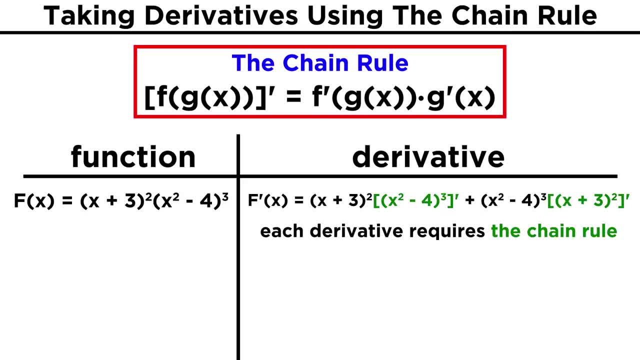 the derivative of the first. But for each derivative we must use the chain rule. so let's expand these portions. For the first derivative, we pull the three out front and change the exponent to a two, Remembering to then multiply by the derivative of what's inside, which is two x. 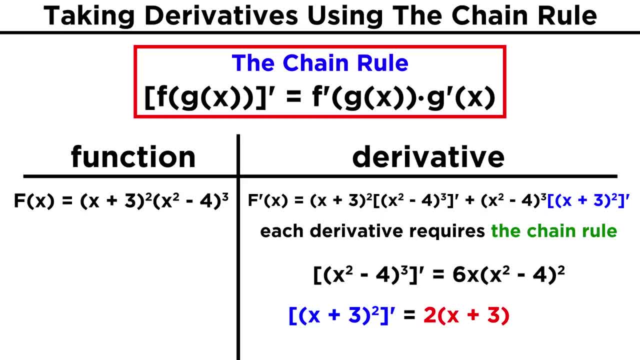 For the other, we do the same thing, getting two times the quantity x plus three, and the derivative of what's inside is simply one in this case. From here most of the work is already done, so let's just simplify a little bit until. 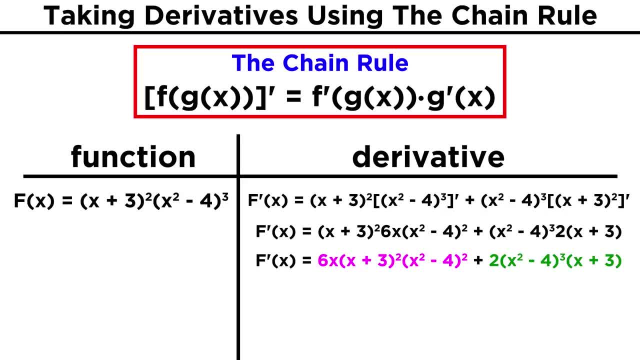 we get two terms. So let's just simplify a little bit. until we get two terms From here, we could identify two terms. We could identify the greatest common factor of these two terms and factor it out, Then just distribute everything that's left inside to get one term, and this is therefore. 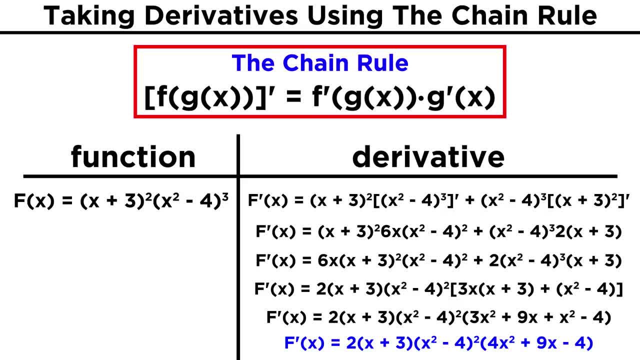 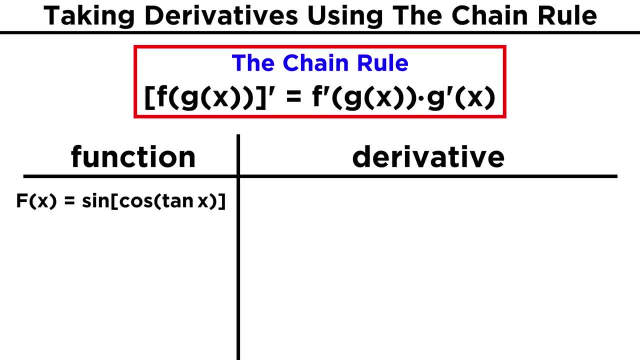 the most simplified way to express our answer. Let's do just one more example to illustrate how crucial the chain rule is. What if we have sine of cosine, of tangent, of x? Let's just apply the chain rule the same way we already have, working from the outside. 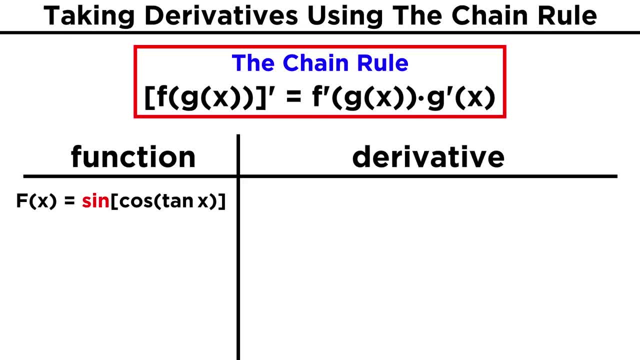 in The outermost function is sine, so let's not worry about what sine is operating on. since that won't change, Just think of it as being equal to u for the time being. The derivative of sine is cosine, so we get cosine of u. 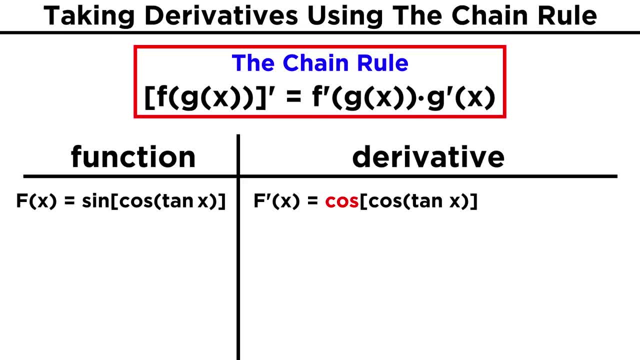 Or the cosine of what was originally in there, so cosine of cosine of tangent x. But then we have to multiply by the derivative of what was inside, and the derivative of u or the derivative of cosine of tangent of x will itself require the application. 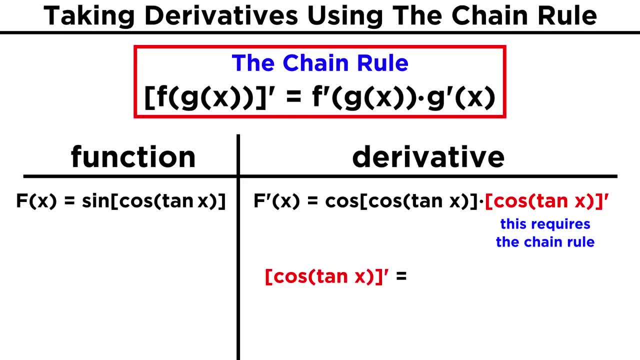 of the chain rule. So let's just keep working our way through this, not touching any of the work we've already done, but now evaluating this other derivative using the chain rule. So let's just keep working our way through this, not touching any of the work we've